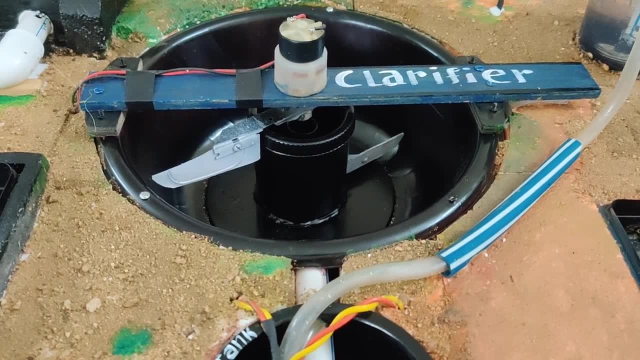 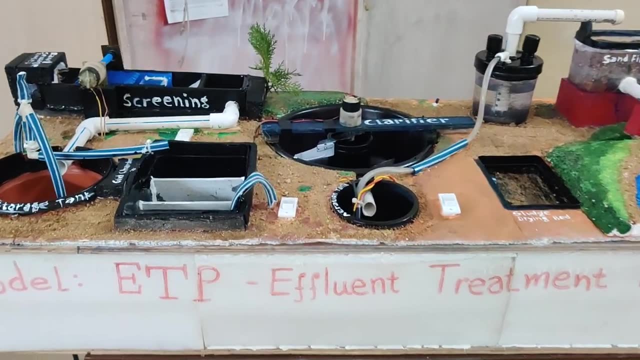 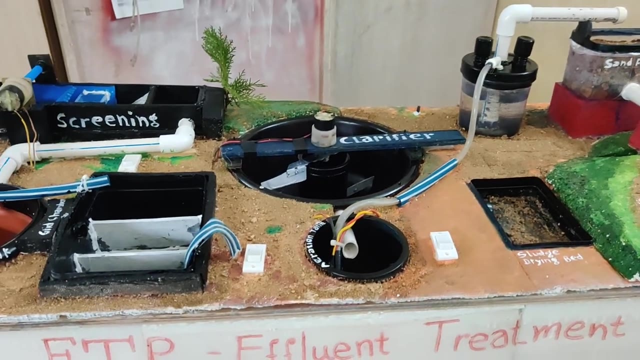 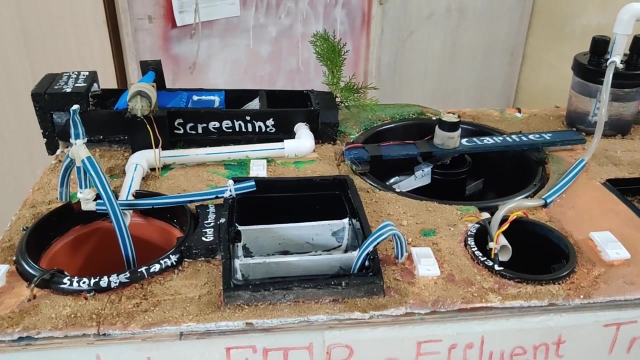 Hello guys, Anang Tata here. This is a model of effluent treatment plant or sea waste treatment plant. I was looking for model of sea waste treatment plant on YouTube and on Google, but I did not get a nice one, and also since I had project for my semester, so 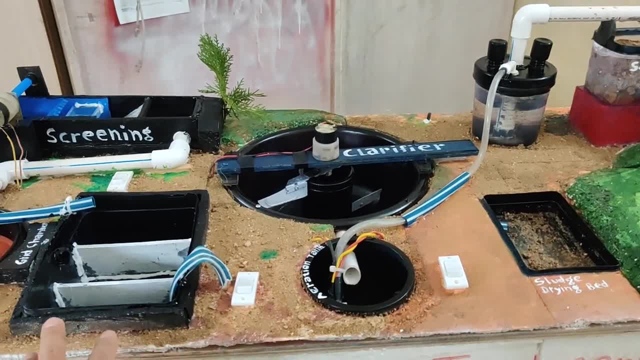 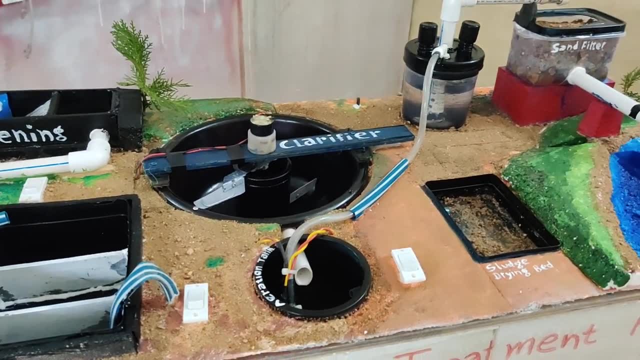 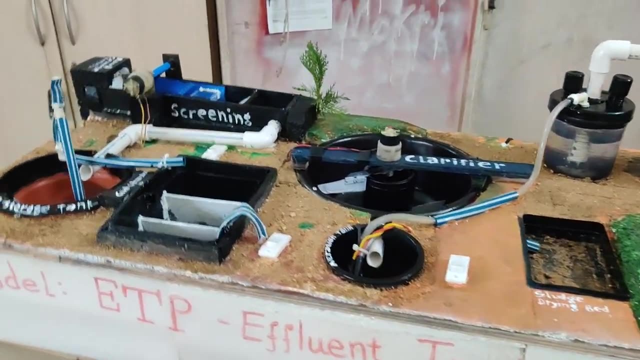 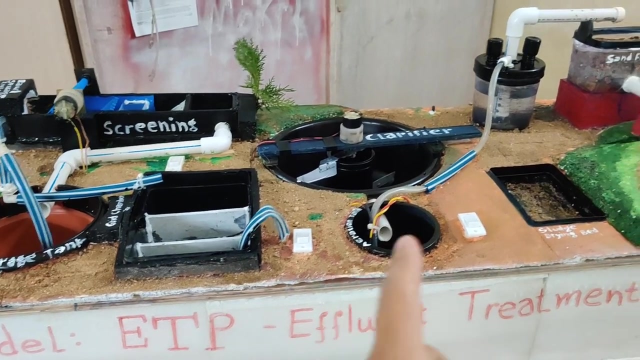 I built this effluent treatment plant. I'm going to share you all the connections and all the pipe works and even the wiring connections, and all so that you can build one for yourself if you're at school or if you're at college. So let me explain about all the process that is involved in here, and I would also like to say that this is the 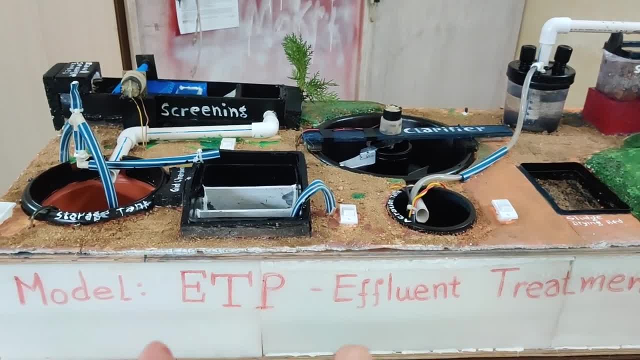 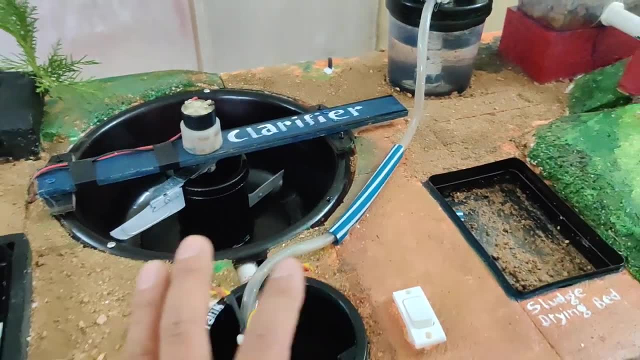 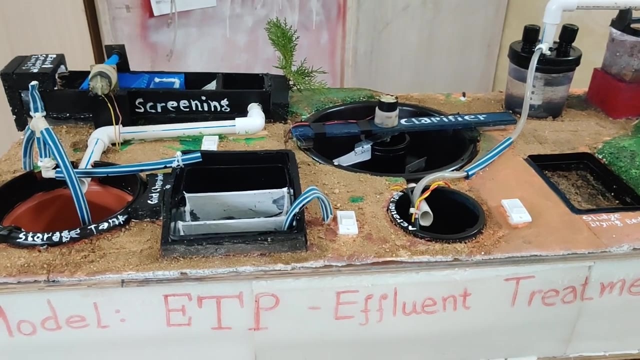 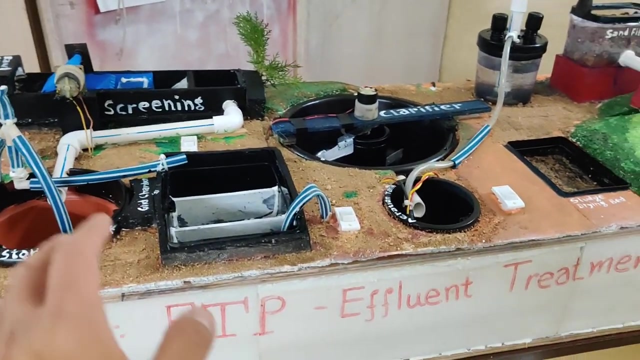 biggest part of a sea waste water treatment plant, since they are like primary or secondary clarifier and all, and depending upon the type of treatment, maybe it's a sea waste water from a dye factory or from industry or local household sea waste. the process may vary, but then in the end it all comes down to treating the water. So I'm going to share you all the connections and all the pipe works and even the wiring connections and all so that you can build one for yourself if you're at school or if you're at college. So let me explain about all the process that is involved in here, and I would also like to say that this is the biggest. 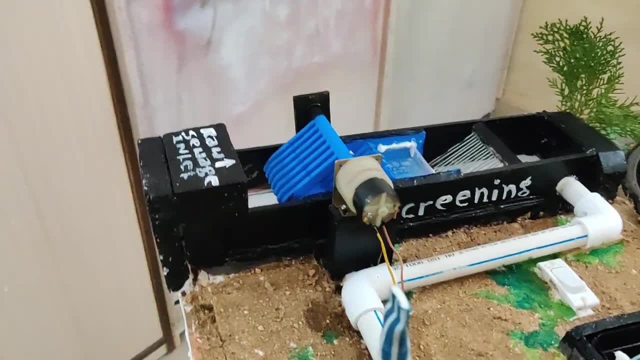 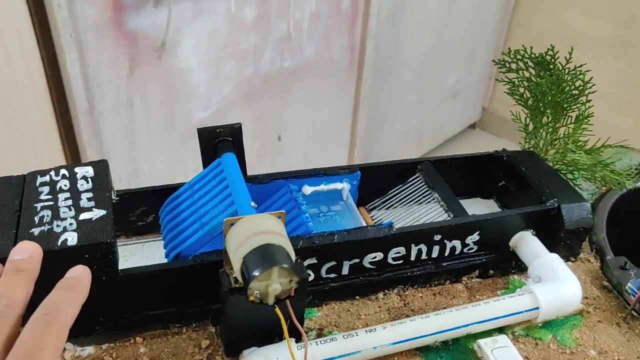 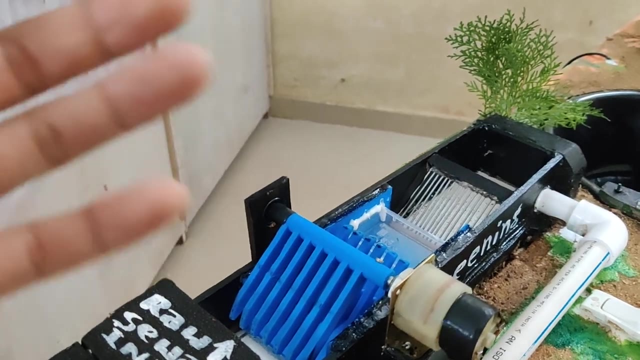 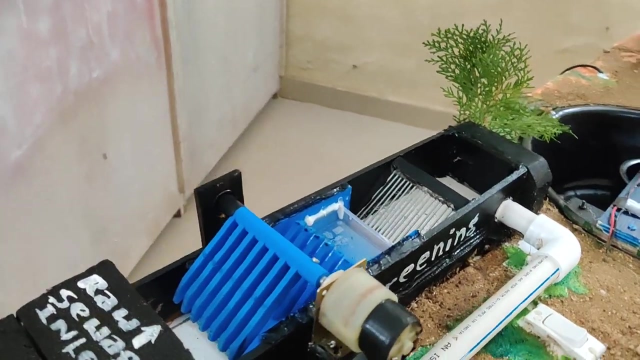 part of a sea waste water treatment plant, since they are like primary or secondary clarifier, and all so that you can build one for yourself if you're at college. So let me explain about all the processes that is involved in here, and I would also like to share you all the connections and all so that you can build one for yourself if you're at college. So let me explain about all the processes that is involved in here, and I would also like to share you all the connections and all so that you can build one for yourself if you're at college. So let me explain about all the processes that is involved in here, and I would also like to share you all the connections and all so that you can build one for yourself if you're at college. So let me explain about all the processes that is involved in here, and I would also like to share you all the connections and all so that you can build one for yourself if you're at college. So let me explain about all the processes that is involved in here, and I would also like to share you all the connections and all so that 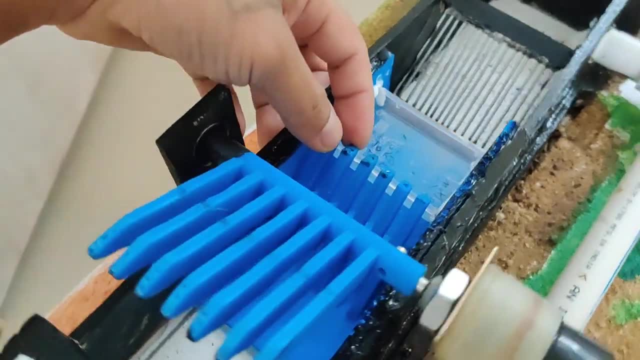 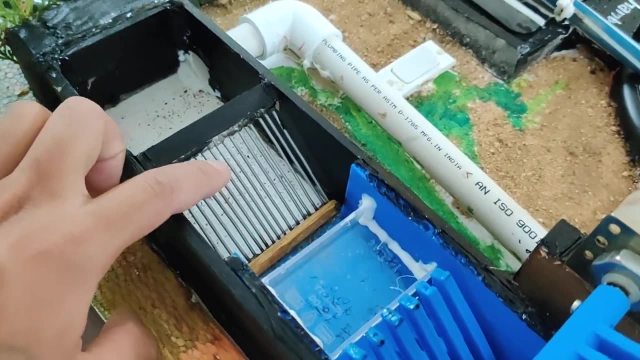 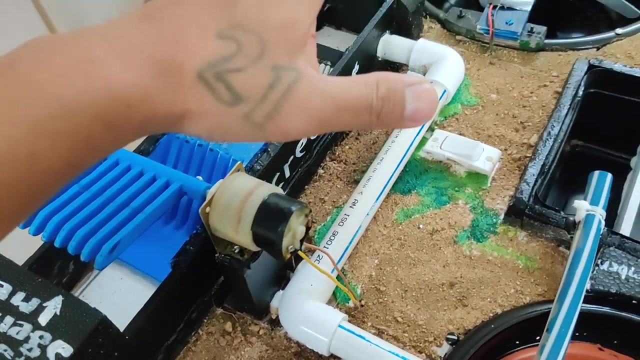 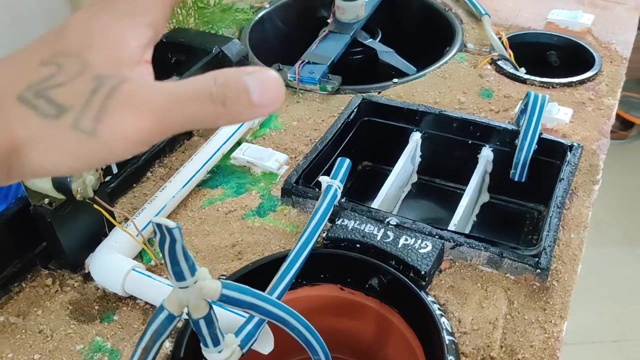 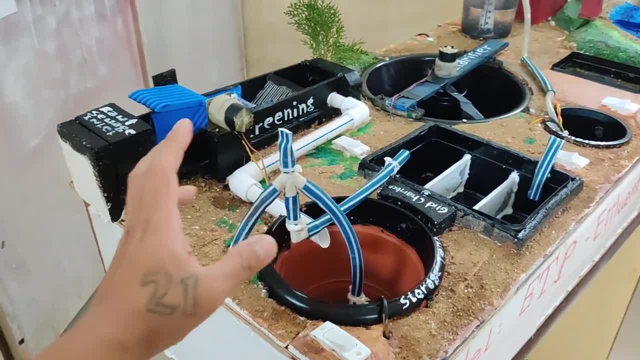 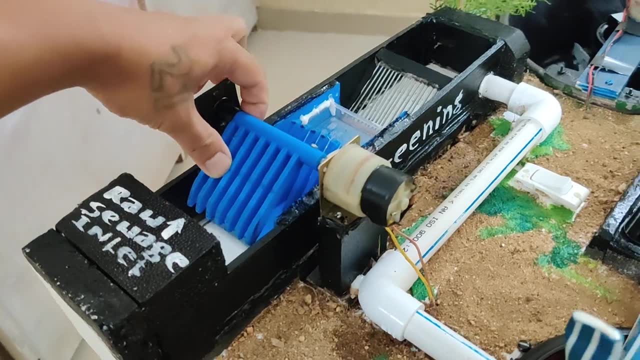 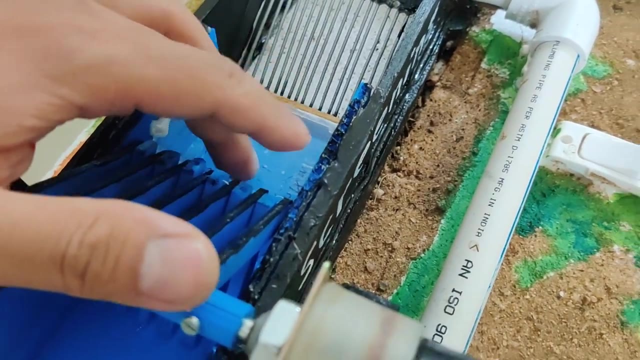 is in this project so that you can- so that you can- make a model of this one yourself. so what does this thing do? is it it pick up the dress or debris and then put it here in this tank? I don't have anything right now, so I'll just use. 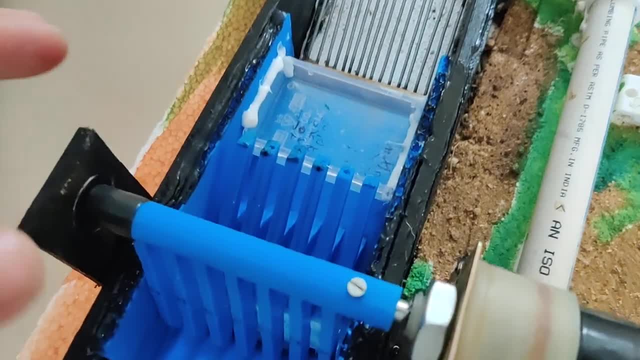 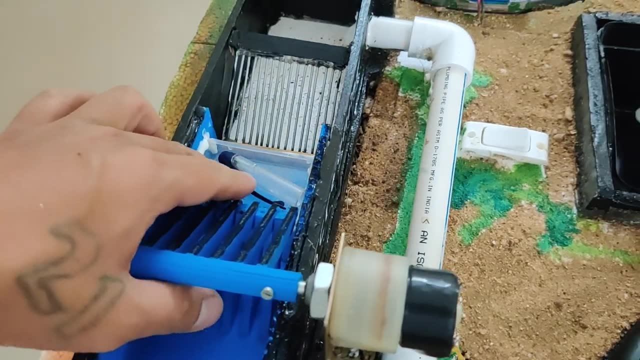 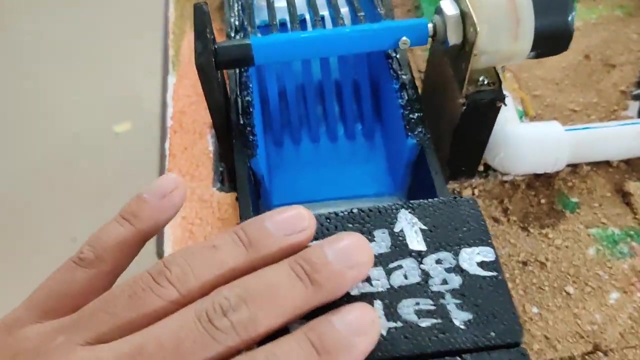 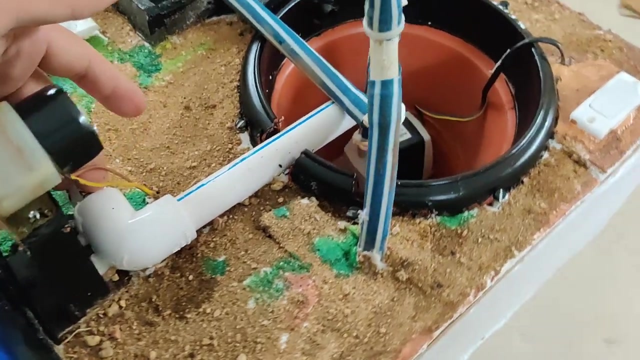 this pen. suppose it's filtered in this grid, and then what this arm will do is it will pick it up and this is like the garbage thing, or whatever you want to call. so from this seabed water it gets into the screening and then all the debris are screened and then the next water is water is sent to. this is a. 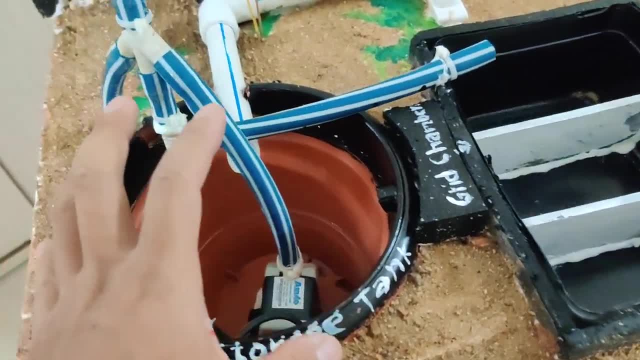 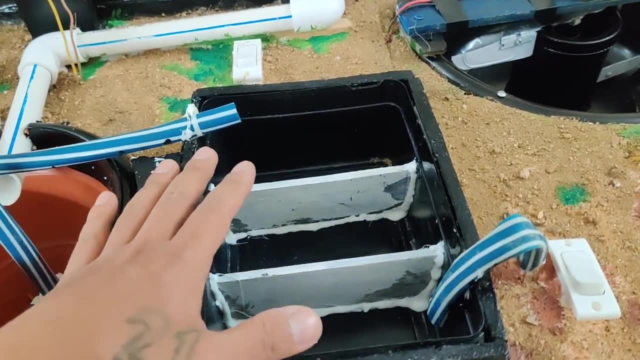 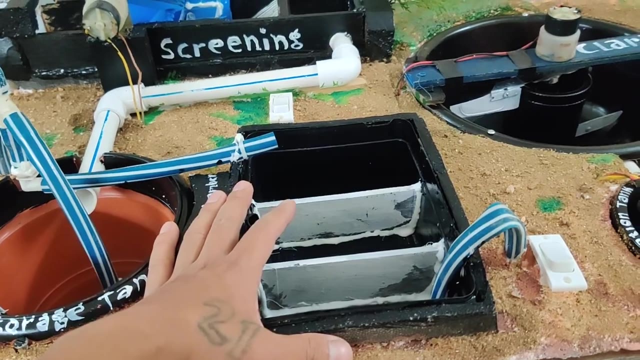 storage tank, so all the seawater is stored here after screening and then it is pumped to the grid chamber. this is a chamber- it's like kind of settling chamber- where the darts like sands or small spables or whatever- is not whatever- passed through the screen, it gets. 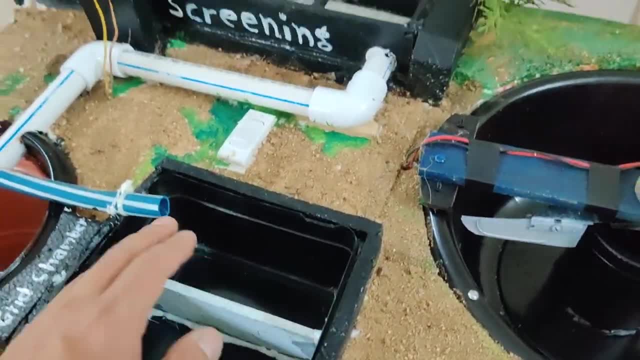 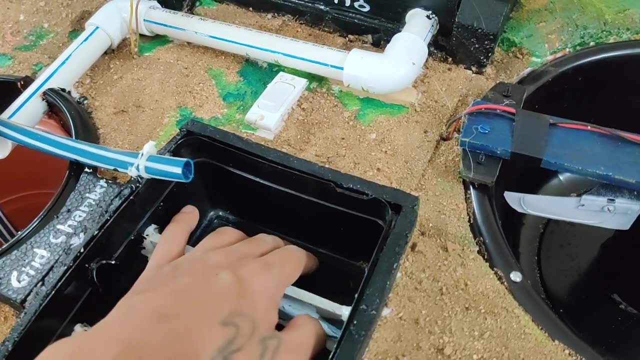 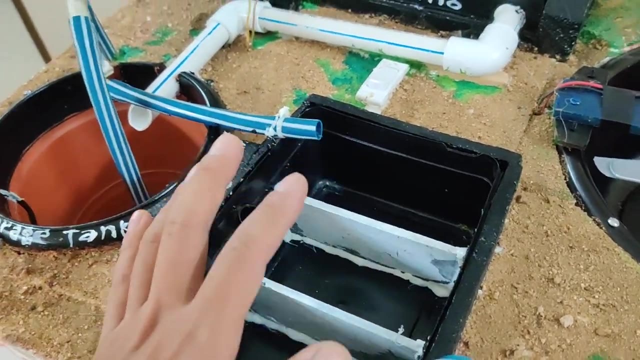 time to settle in this thing. so we have three partitions here. first the incoming water flows here and then it gets enough time to settle on the heavier particles, and then next we. next it goes here and by the time it reaches here like it gets enough time to settle down. so once all the grids 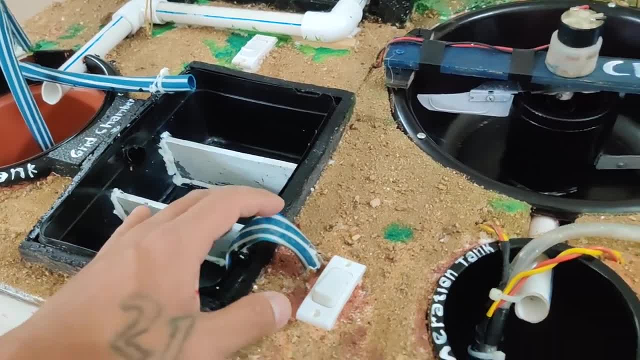 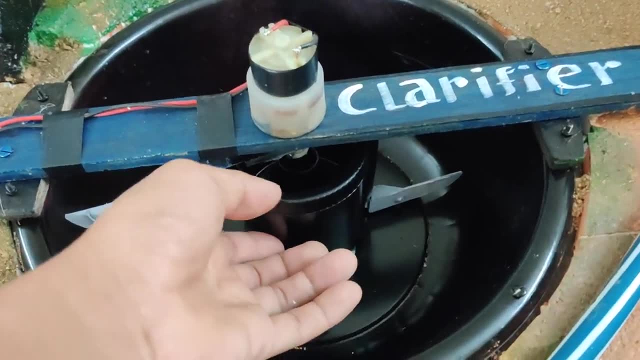 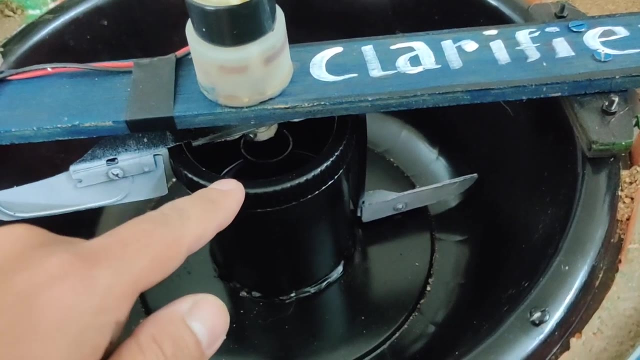 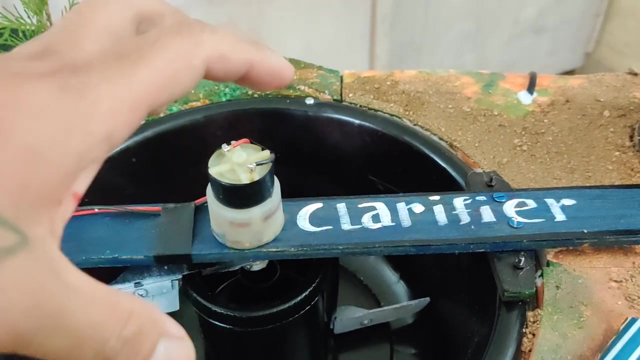 are settled down. next, the water is pumped into the clarifier tank. so water goes inside in the clarifier tank. we have this bigger diameter tank and then smaller one, and then- this is also important- it is like it, like it diffuses, or diffuses the turbulent of the water. so water comes from this smaller, 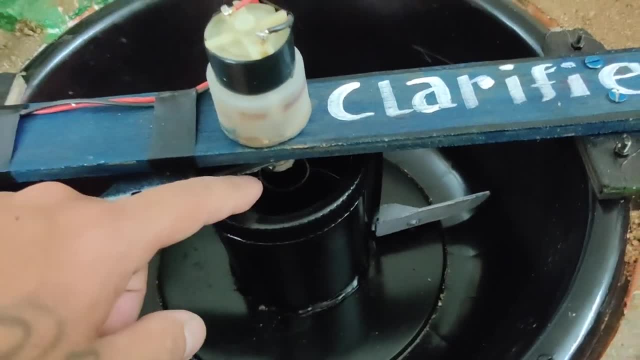 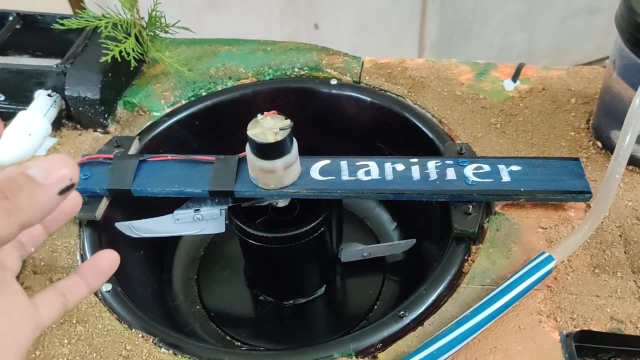 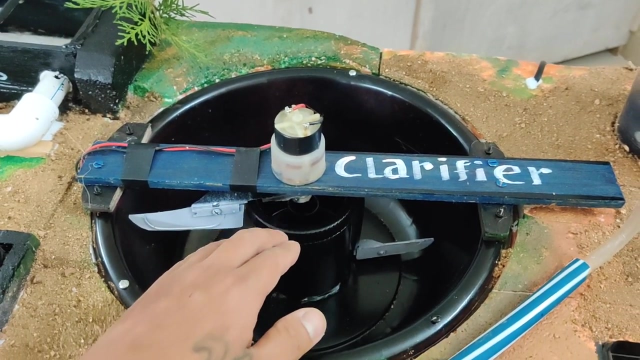 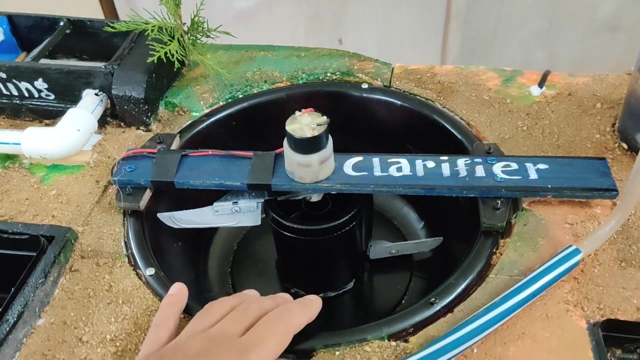 pipe. and then here we add the coagulants and all like alum so that the suspended- suspended what you call darts- may be settled down and water overflows from here. it's overflows slowly into the, into this bigger tank, and since it gets lots of time to settle down, so most of the 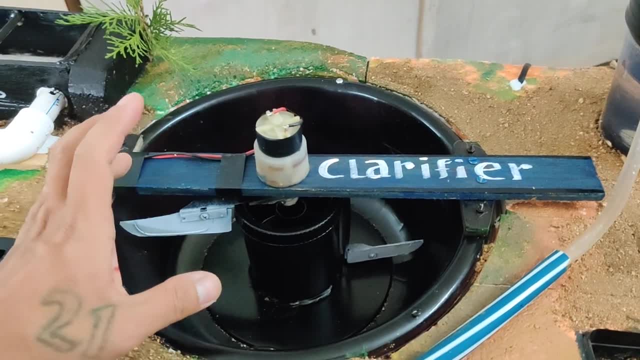 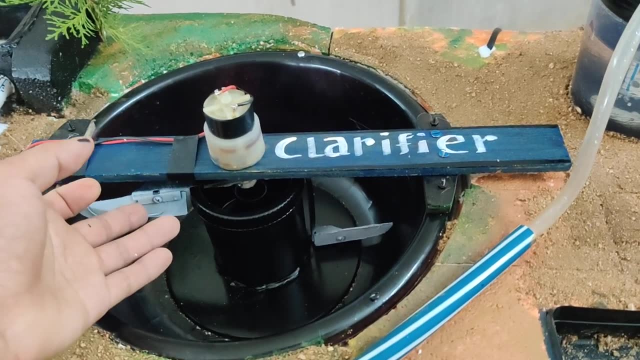 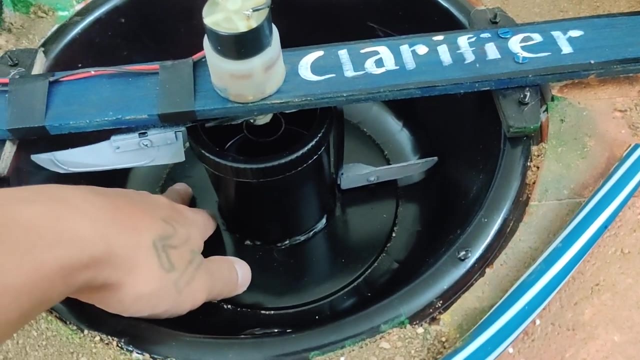 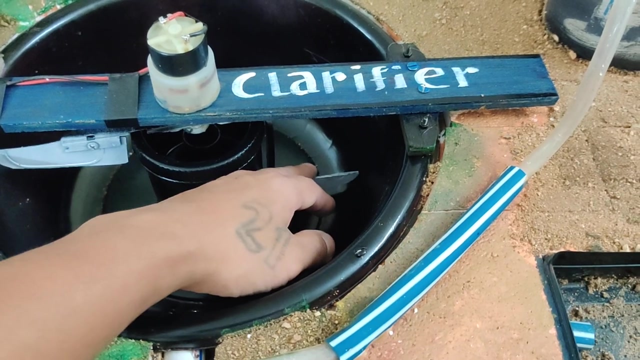 coagulants are settled down here. i mean after the proclamation. so in this grid: clarify: we have this coagulant. so in this grid, i clarify: we have this coagulant. this is a scraper. once all those, once all those darts are settled. this thing, it rotates slowly. 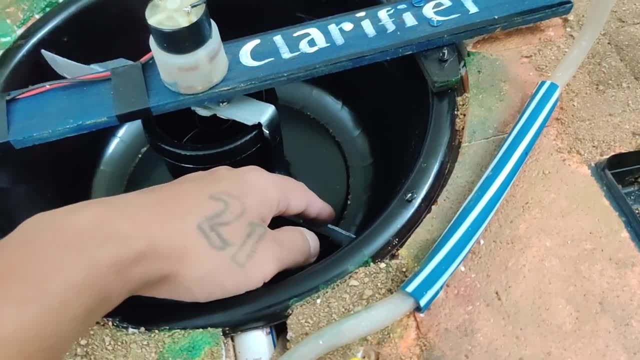 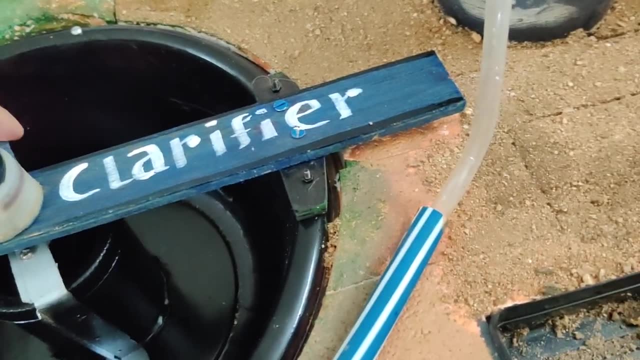 and this: this is the scraper which scraps the darts and send it to the slice speed. and also on top of that, we have the just a second. this is, this part is a screamer. and also on top of that we have the just a second. this is this part is a screamer. 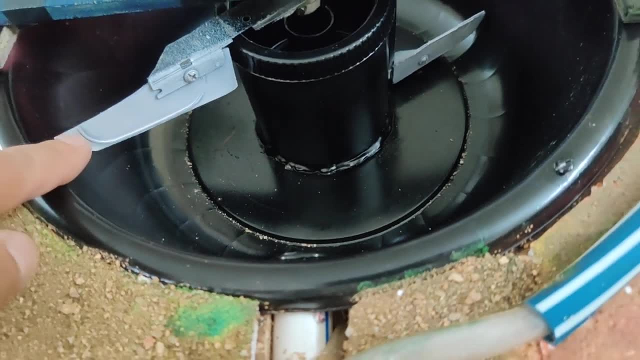 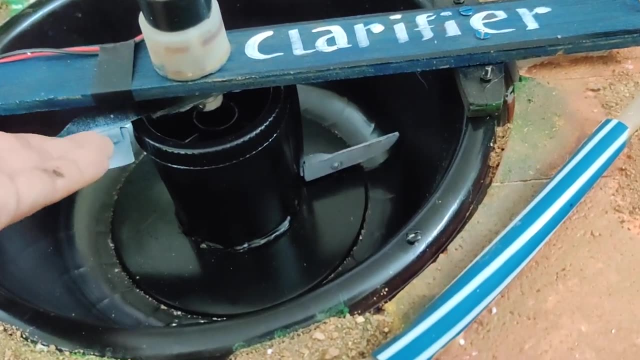 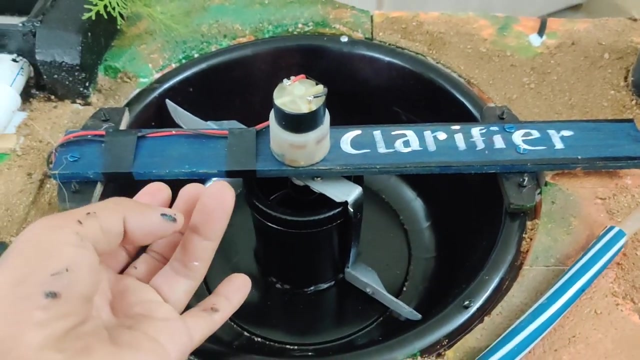 water is. water levels is up to this much, water fills up to this much, and then anything that floats like oils on any other thing, any other darts. it gets skimmed here, so the heavier particles settle down and then the lighter particles. uh, like what do you call? 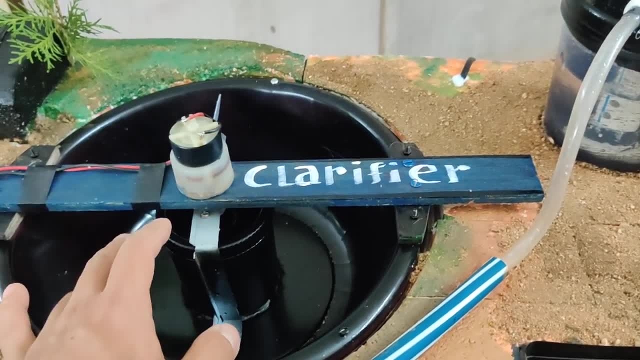 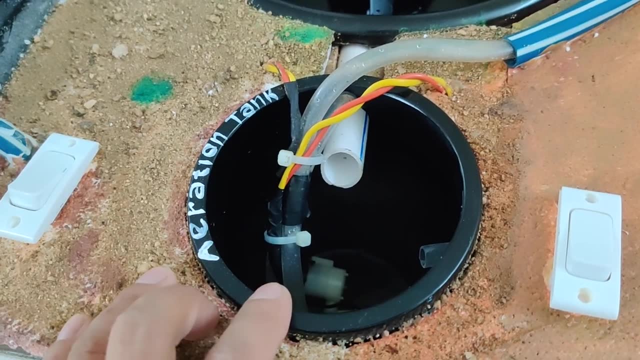 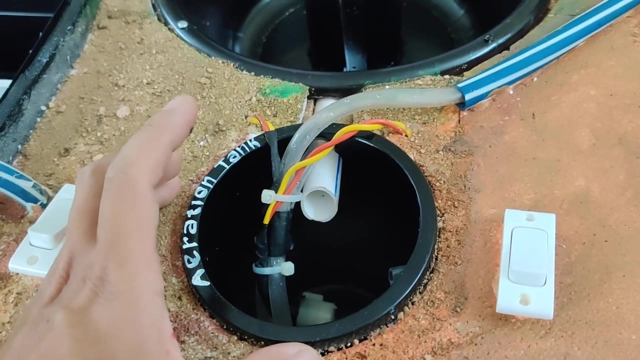 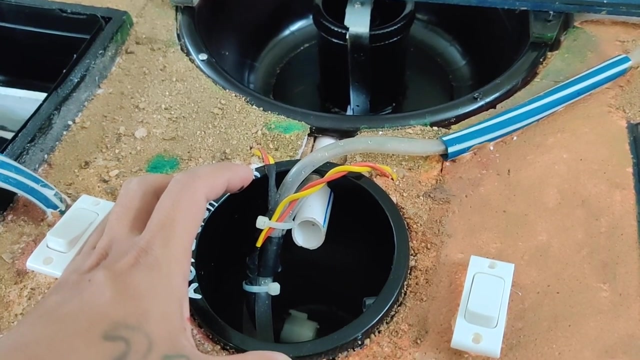 it. it is skimmed by the screamer and then after that, uh, the water overflows into this another tank. this is a recent tank. here we supply lots of air, and then anything organic is decomposed by the anaerobic bacteria- sorry, aerobic bacteria- with the help of oxygens. so after this, actually there should be one more. 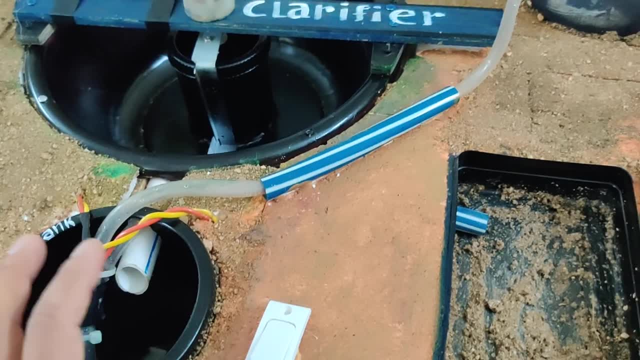 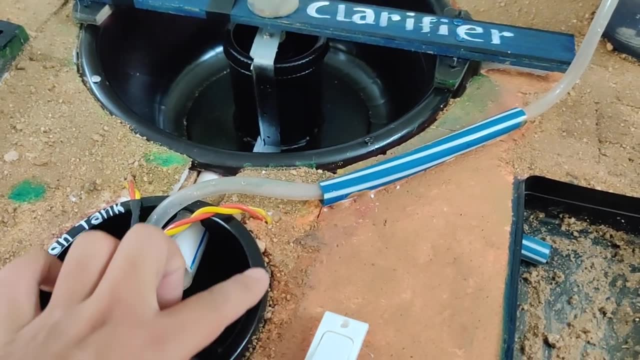 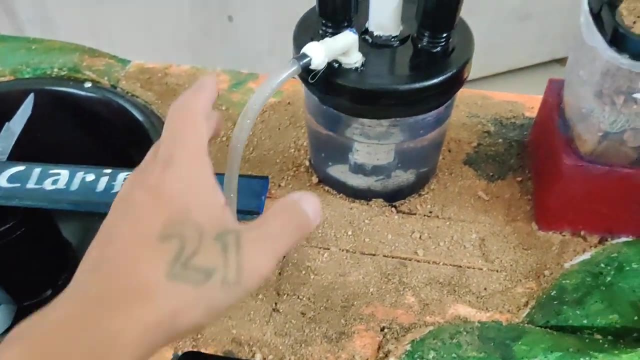 clarifier thing. but then we don't have lots of space and then i, for the sake of explaining the process, i'm going to just include this one. after the aeration tank, most of the cleaning is done here, and after the aeration thing it goes to the water, is pumped to the disinfection tank. here we 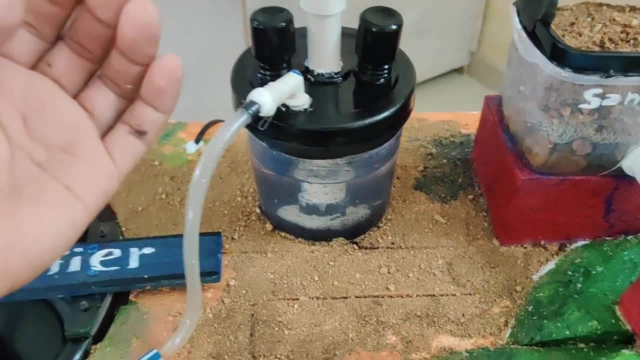 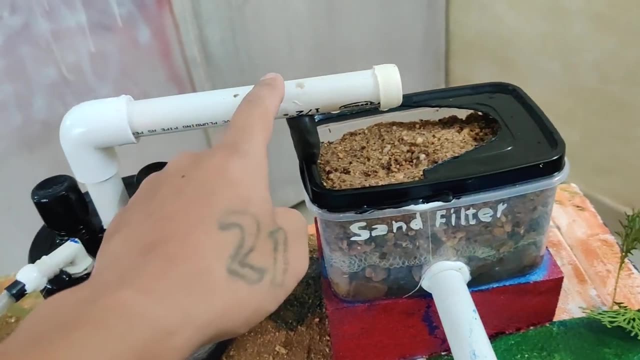 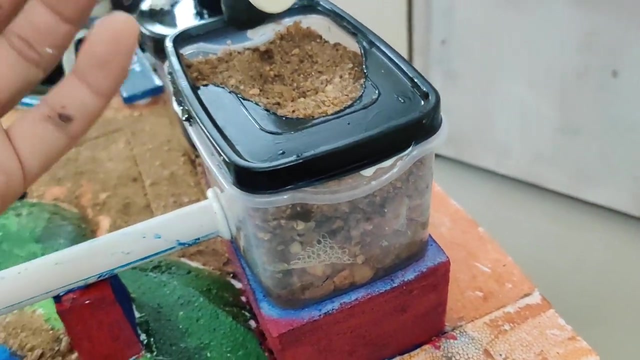 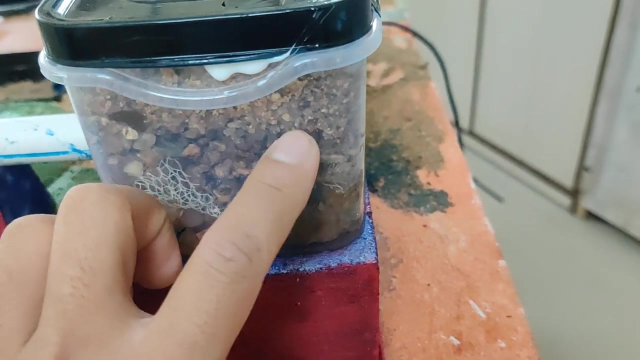 get disinfections like chlorine and all, and then from there the water is pumped or passed into the sand filter. the sand filter, it's like it's a process for filtering the water from bacterias and all. so we have different, different size, uh, of saints and stone and all on the top. 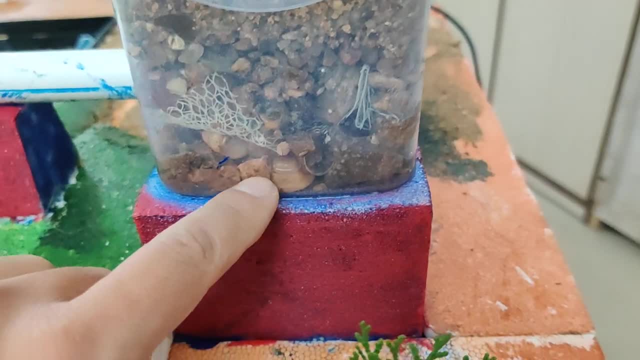 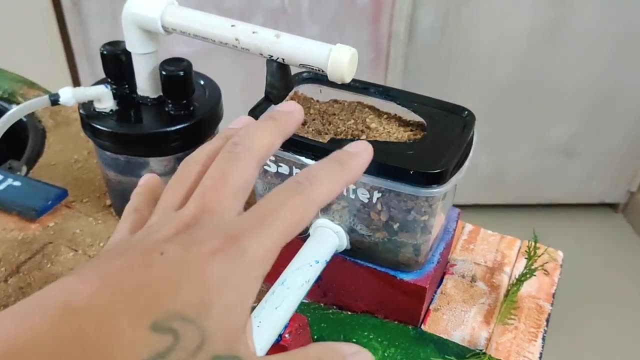 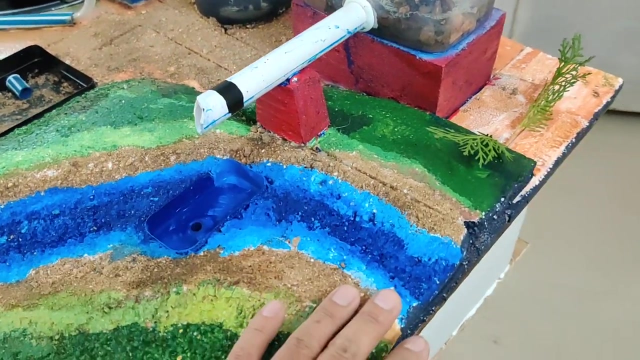 we have the smallest one and then, as we go bottom, we have the bigger one there. so from there, from the sand filter, uh, the treated water. after all this process, most of the water is cleaned and it is discharged into the river and this project, it's a closed loop. 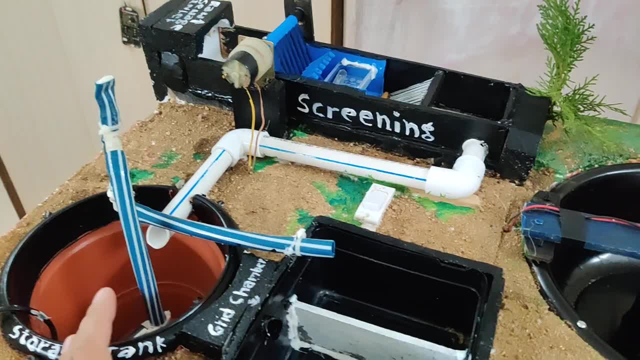 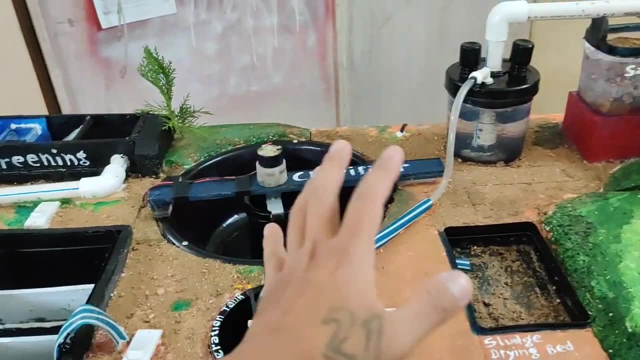 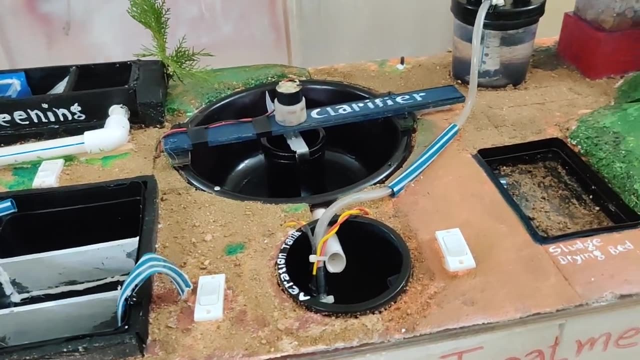 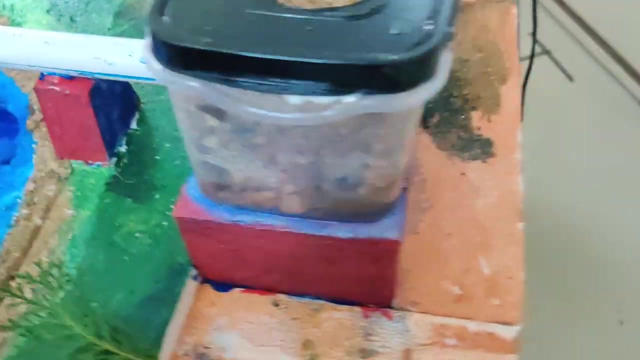 circulation. so what have? what is happening here is like: once we put the water, it is cycled. throughout this project- i mean this throughout this model. so this is a closed loop, closed circulation system. so even the discharge water, it goes into this pipe and then we have another. 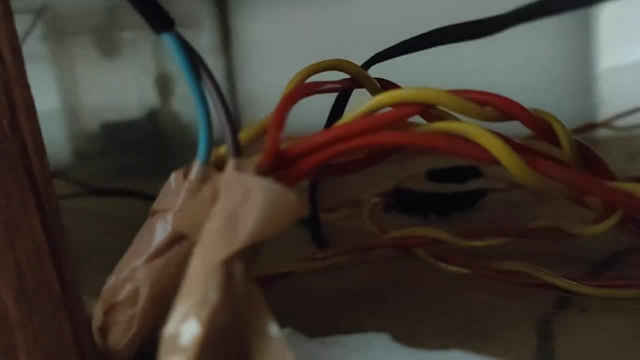 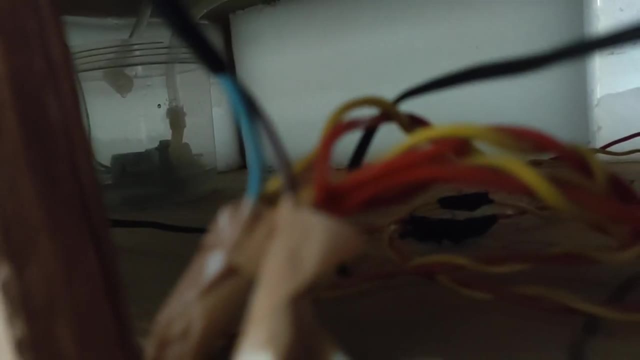 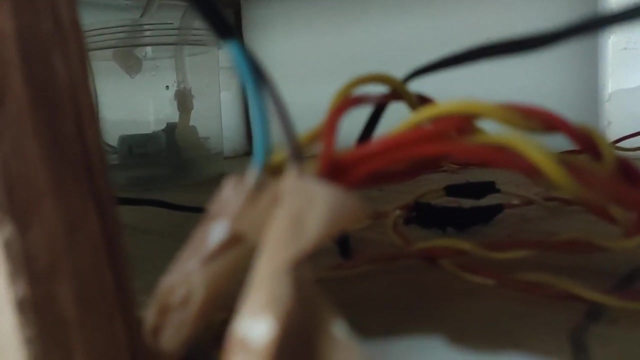 now let me- i don't know if you can see it. yes, we have another thing there with motor pump, water pump. so the water from the river it is discharged into the tank and then it's since this is a closed circulation system, so it's again sent back. 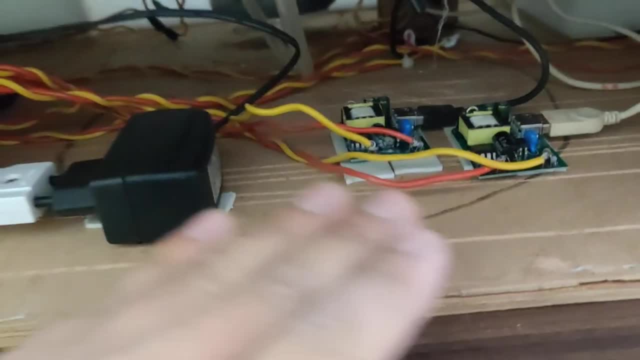 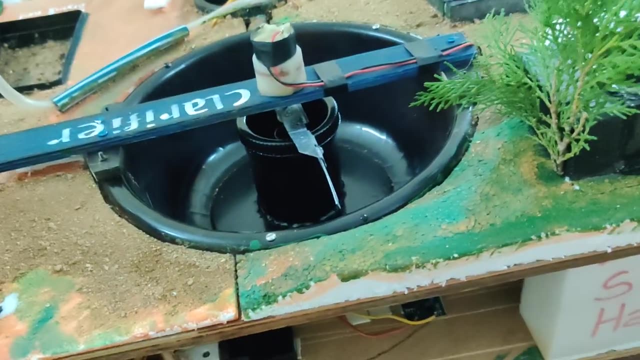 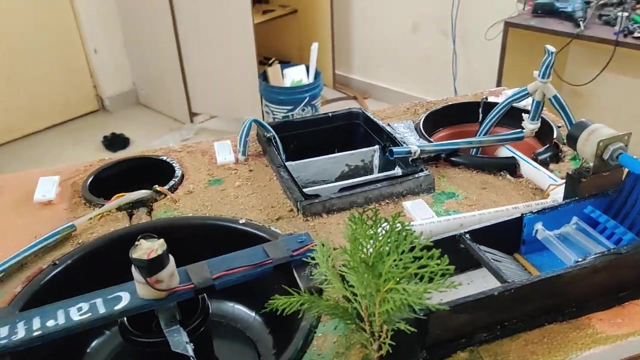 to that aeration thing for now. and these are the power supplies. we have different power supplies because there are lots of different, different motors. some are powered in 5 volts and some in 12 volts and some even in 120- sorry, 220 volts. so this is a complete process of